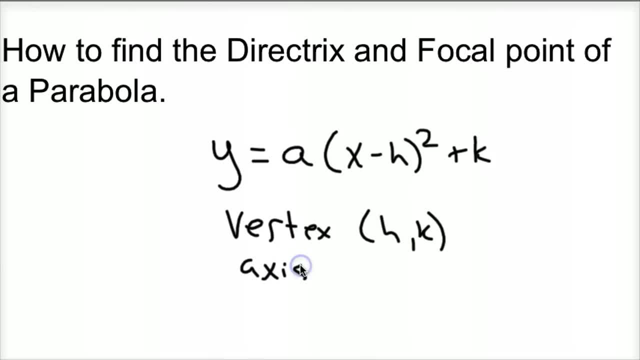 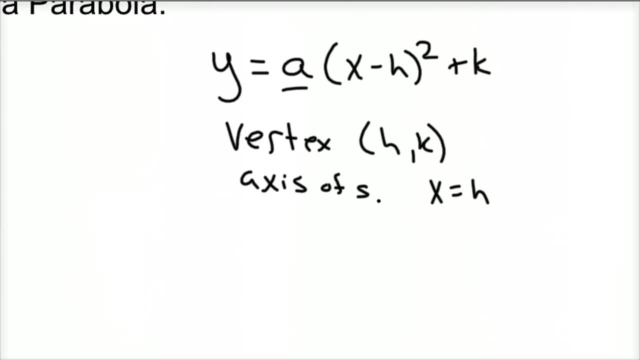 And our axis of symmetry- I'll just call it axis of s- is the value x equals h, And a told us how wide or narrow the graph is. Well, that also happens to determine where your focus and directrix lie, And so, what you can do for focus and directrix, let a equal 1 over 4p. 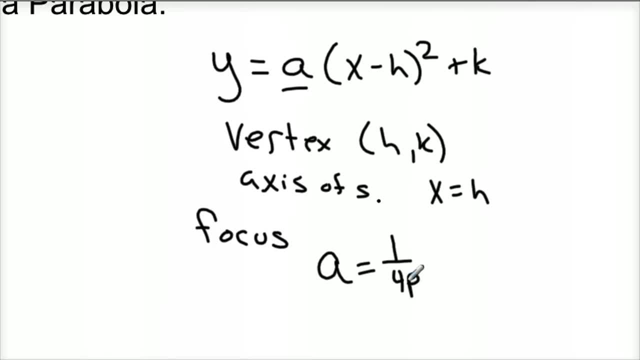 And that value p, then let me kind of just show you what that is. So if you had a parabola here and p is this or this is your focus, we'll call it f. So this distance here to the vertex is p. 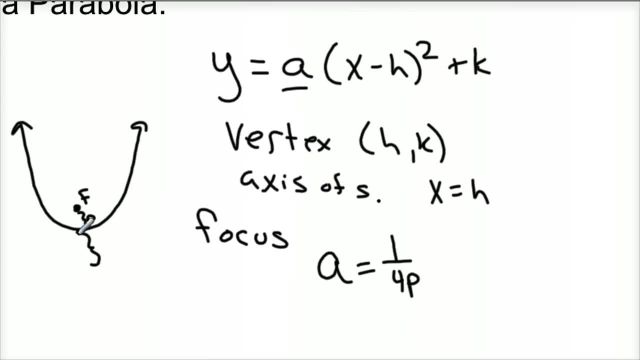 And then that exact same distance from the vertex down is your, that value p, And p is also to your axis of symmetry. So that is how you find it. So you could, you know you could multiply this out and come up with a formula for it. 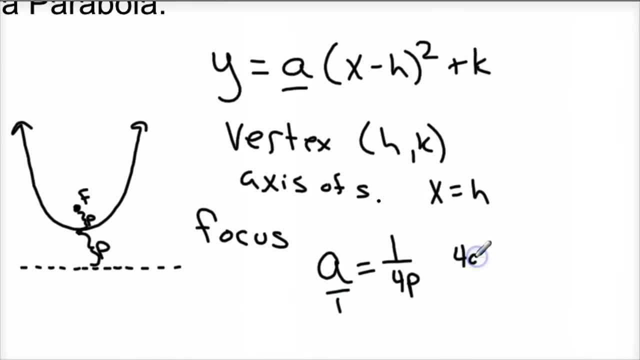 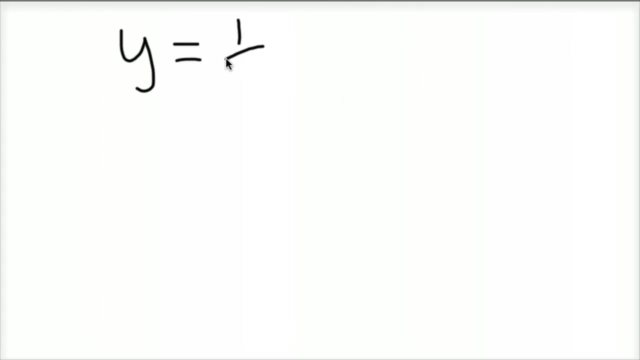 This is a over 1.. So 4ap equals 1.. So p is equal to 1 over 4a. So that will tell you your distance to your focus from the vertex. So let me give you a couple examples. So let's say we had y equals 1, fourth x minus 3, squared plus 2.. 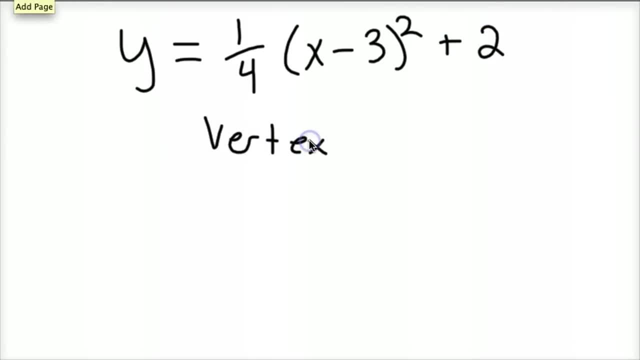 Okay, so we know the vertex is 3, 2.. We know our axis of symmetry is x equals 3.. And we know our focus and directrix can be found with the equation: 1. fourth equals 1 over 4p. 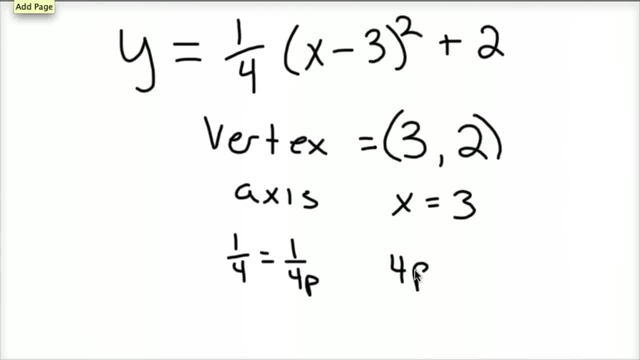 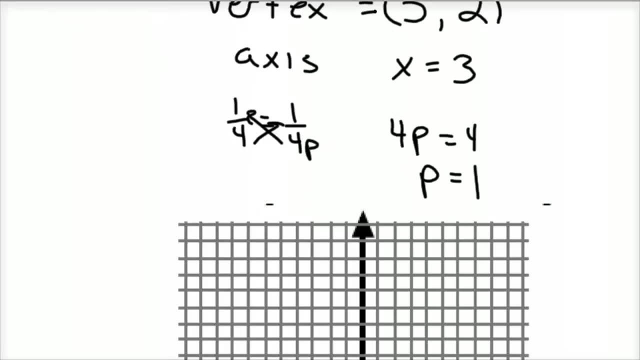 So if we cross, multiply that 4p equals 4.. So I know my value p is 1.. So that tells me when I graph this thing. So when I graph this thing I've got 3, 2.. So I've got 3, 2.. 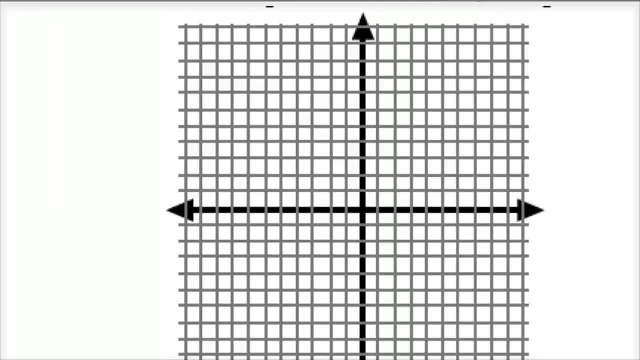 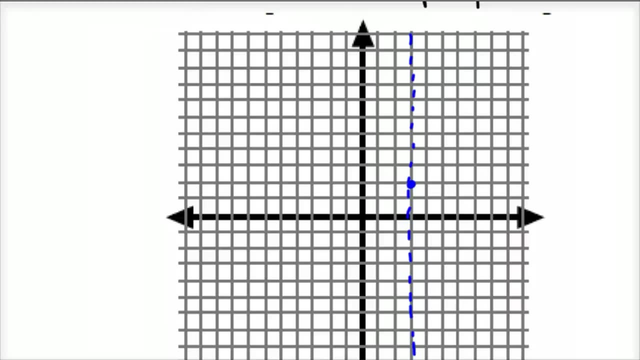 So I'll graph that. So there's my vertex. x equals, 3 is my axis of symmetry, And p then is 1.. So I'll put that in red. So that means from my vertex. since this is a happy graph, I'm going to go up 1.. 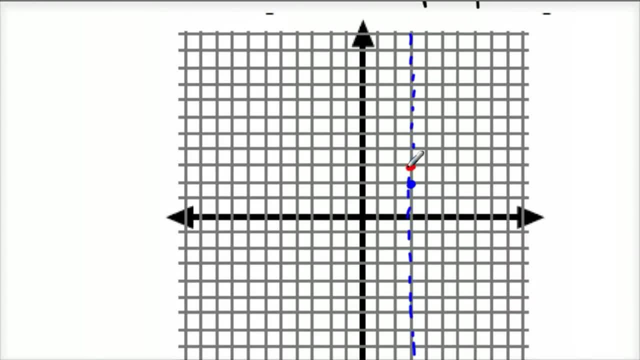 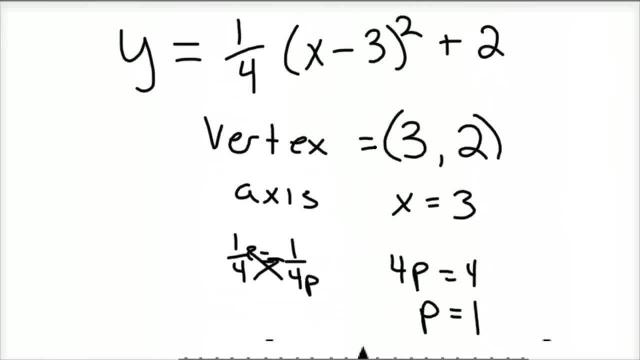 Because the 1 quarter is positive. It means it opens up, And if I go down 1, I make a point And this line is my directrix. Now, the special thing about a directrix is- and let me go back to my original kind of rough sketch drawing of that- 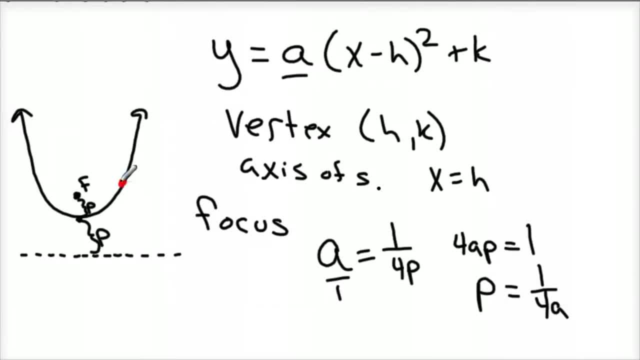 A directrix. if I have some point out here and I draw a line from the focus to that point on the parabola and then down at a 90 degree angle. these two values are the same distance here and here. 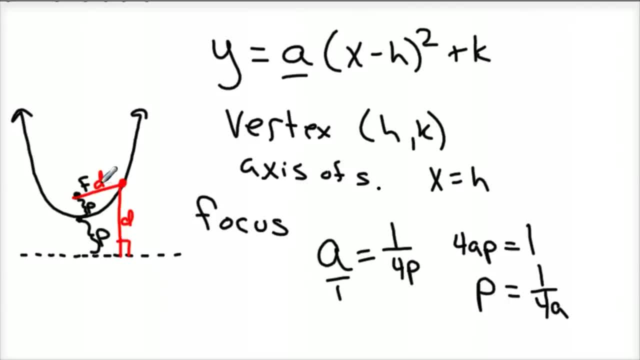 So that's the special thing about a directrix. So no matter where I'm at, so even if my point was up here, so my focus to that point, then straight down to my directrix. these distances are the same. So maybe this one's A, that means this one has to be A. 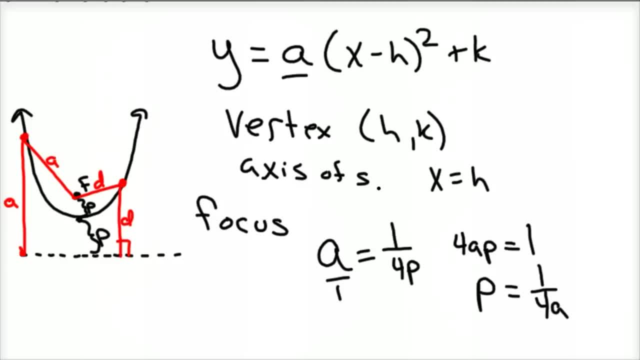 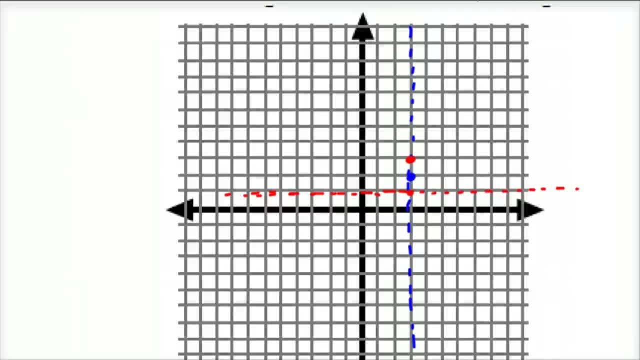 And so that is the special case for a directrix and why it's so important. So one of the reasons why it's so important. So now you know, we're getting to the point where it's probably time to start getting around the same result. 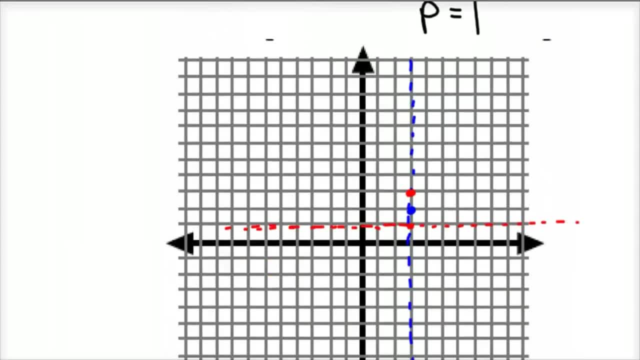 So let's get started getting a few more points for this thing. so I'm gonna pick, pick another point. so maybe- oh, I don't know well, let's do 0. I always love to plug in 0. so this is X, this is Y. we'll plug in 0 into that function and so you would have negative. 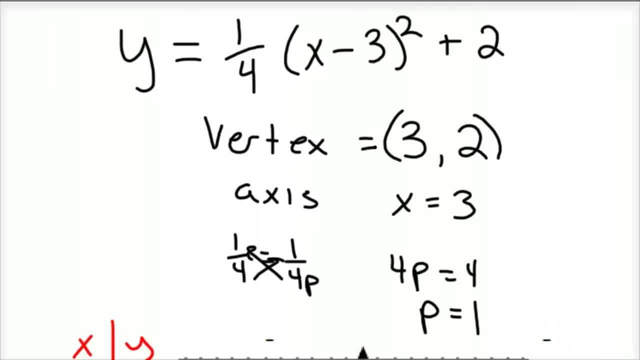 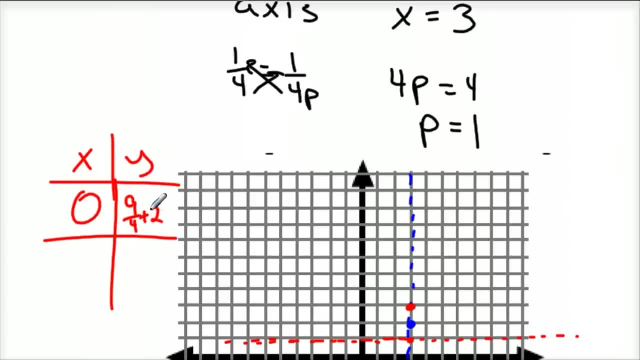 3 squared, which is 9, 9 force plus 2. so let me put that up here: 9 force plus 2. well, 9 force is 2 and 1 fourth, so this is 4 and a fourth, so 0 comma, 4 and a. 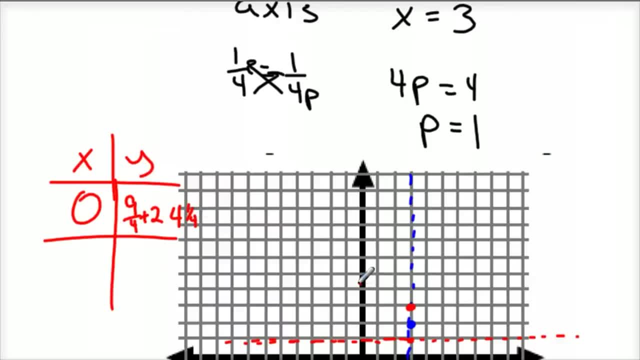 fourth: 1, 2, 3, 4 and a fourth would be right there. then you can use your axis of symmetry. I should be doing that in blue. you can use your axis of symmetry to mirror that. so this is 1, 2, 3 to the right, 1 2, 3 to the left. so I know. 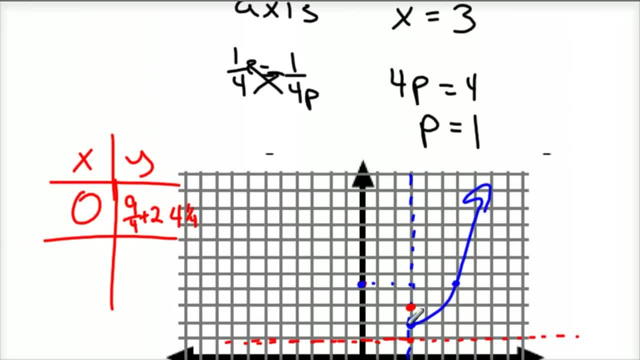 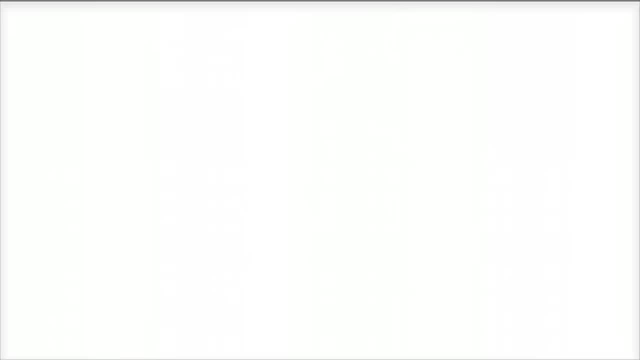 another point has to be there, and we've got a pretty good idea of what this graph looks like now. so that's that particular graph. what happens if you have? what happens if you have something that's solved for X? so let's say you have X equals 1, 8, y plus 4, squared minus one? 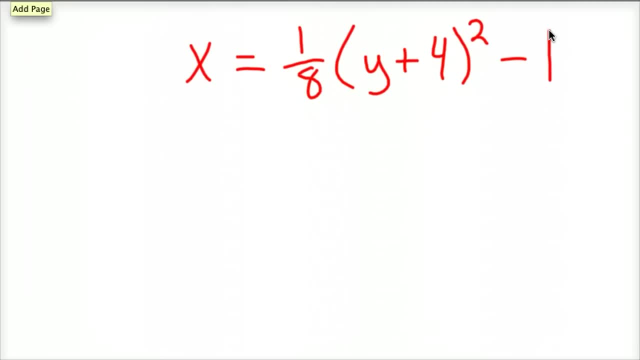 ok, Okay, so back. you know previously we knew what those I'd already talked about: how to find the vertex for this. This is a graph that is- let's make it negative- 1, 8.. So this graph actually is going to open to the left instead of up and down. 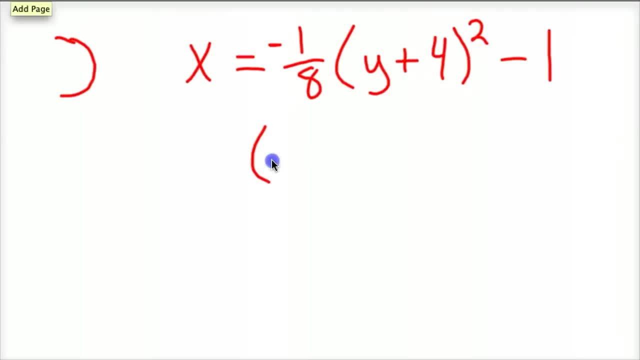 And so when you graph this, negative 1 is my x value, negative 4 is my y value, Because you change the signs coming out of the parentheses there. And so, and my axis of symmetry is y equals negative 4.. 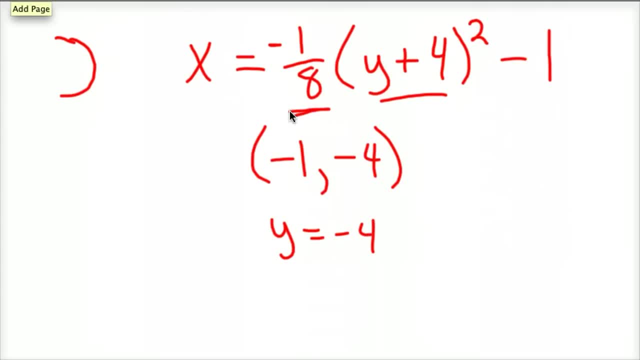 And, just like the previous graph, this a value, determines where your focus lies, Not foci. there's not more than one of them, So you'd have negative 1. 8 equals how? 1 over 4p? jeez, stuttering a little bit. 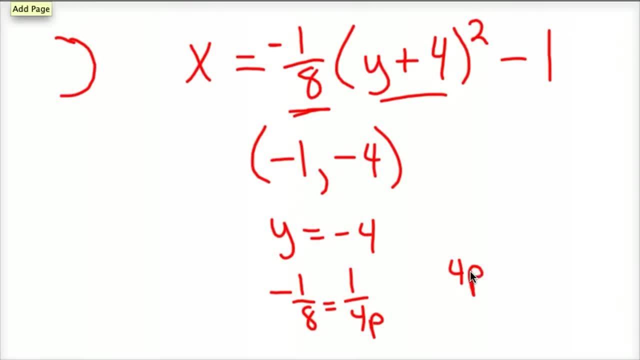 And so you cross, multiply, and so 4p. and we're kind of- since p is a distance, we're going to ignore the sign for now. So 4p equals 8, and so p is equal to 2.. 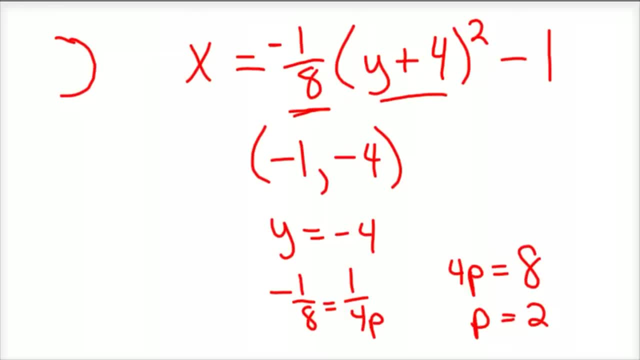 So that means the distance to my focus from the vertex is 2.. But since it's negative and we solve for x, so let me get the graph up so we can have a graph of this thing. Okay, so negative 1, negative 4 is my vertex. 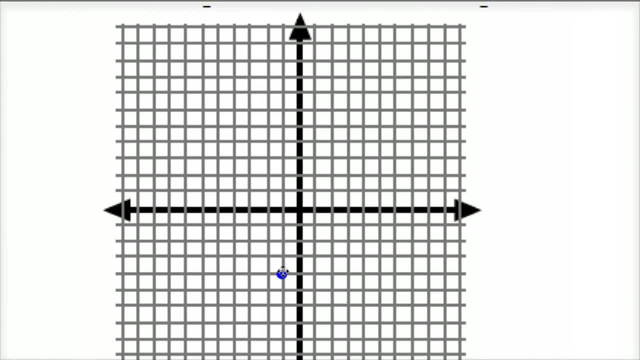 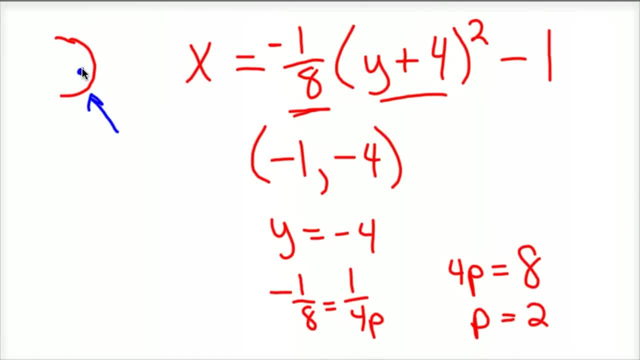 There we go And it's a negative 1, 8.. So I know it's going to open to the left like this. So my focus is going to be here, my directrix is going to be here, And p tells me 2 is the distance from the vertex. 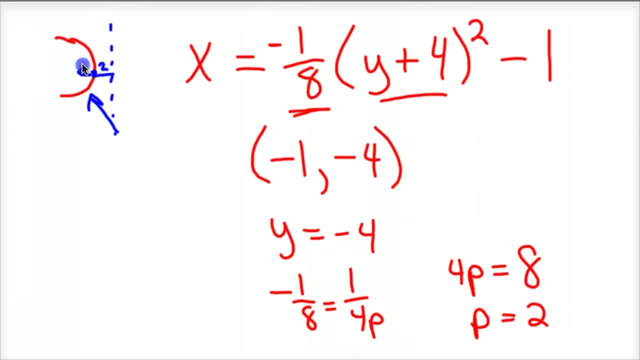 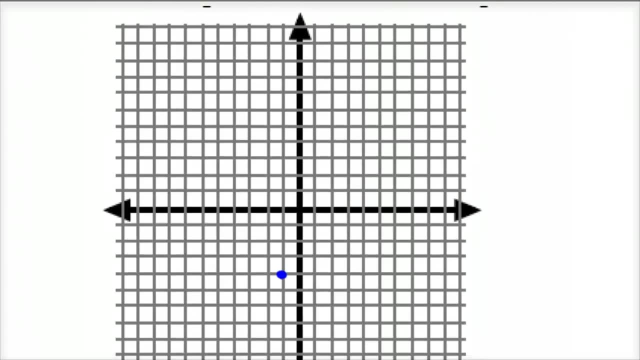 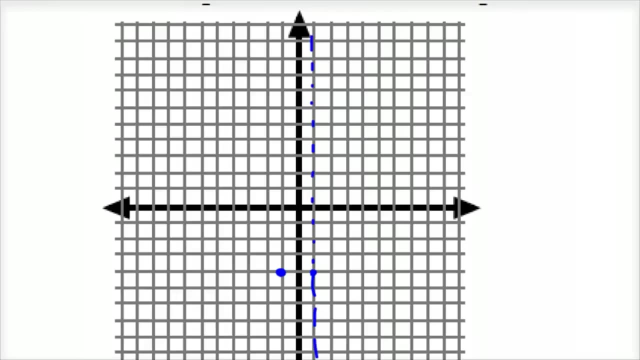 So this distance is 2, and this distance is 2.. So let's go ahead and put that in our graph. So 2 back is right here. That's going to be our directrix. 2 forward is our foci, that's here. 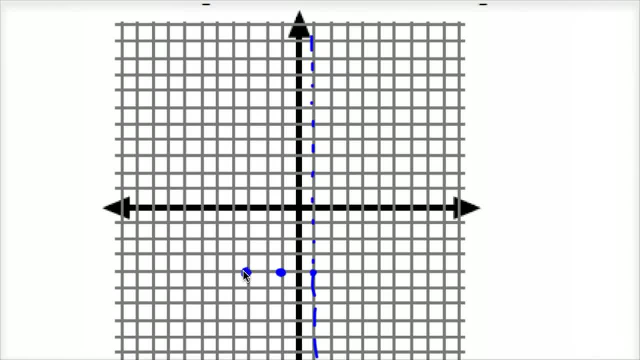 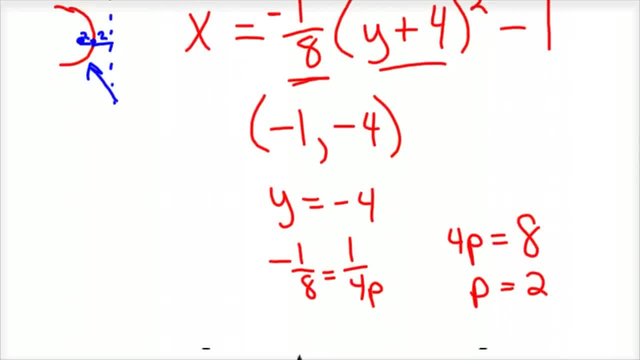 And we're kind of ready to graph some more points on this thing. So maybe let's do. let's see we drew a negative 8.. Let's do: y is 0.. Yeah, So let's put in a 0.. 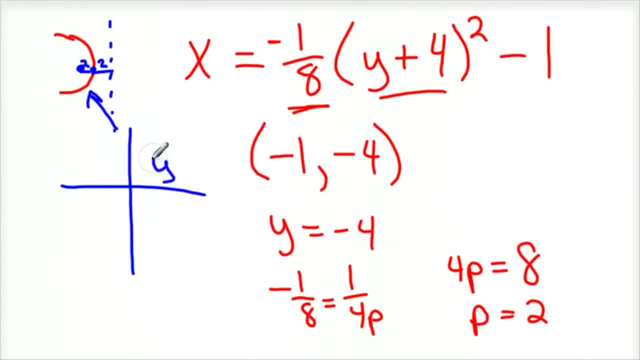 I'll just make a little table right here And we're going to put in for y, we're going to stick in a 0. And see what ends up happening to x. So when you put a y in for 0,, 0 in for y, 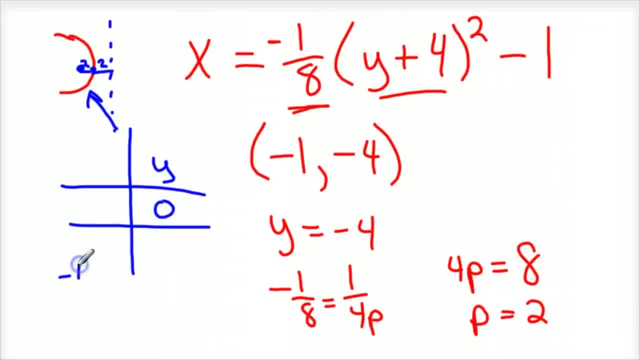 you'd have. I'll put that here: negative 1, 8th times 0 plus 4 squared minus 1.. So that's 16 times negative 1, 8th, Using my order of operation, And then minus 1.. 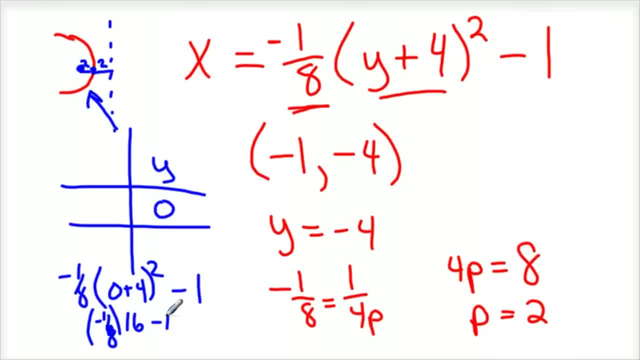 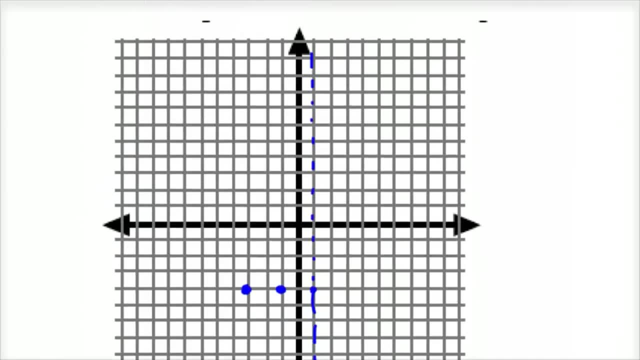 Well, negative 1 8th times 16 is negative 2.. Negative 2 minus 1 is negative 3.. So my x value is negative 3, 0. And my y value So negative 3, 0,. 1,, 2, 3 would be right there. 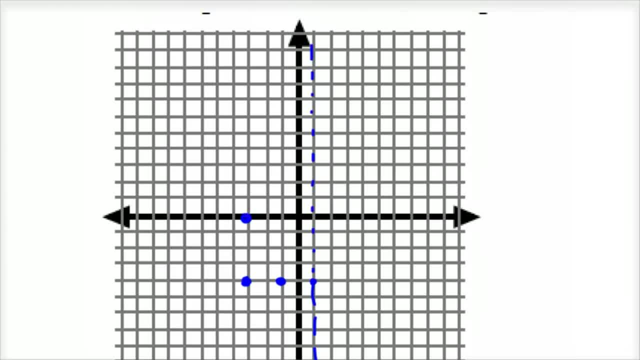 And so you can mirror that across my axis of symmetry, which I forgot to put in. There's my axis of symmetry. I don't know why it curved up like that, but get rid of that one, And so any point can be mirrored across that line. 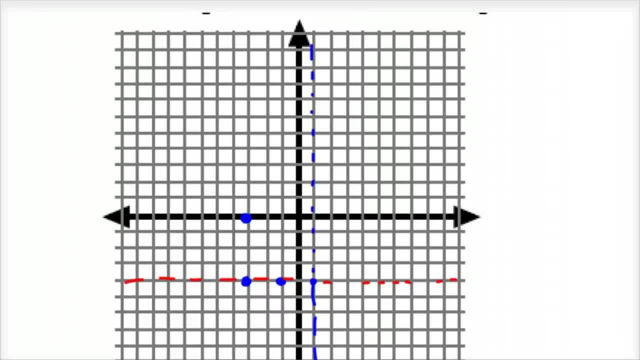 or reflected across that line. So 1,, 2,, 3, 4,, 1,, 2,, 3, 4, would be my axis of symmetry, And so here is what my graph looks like approximately.